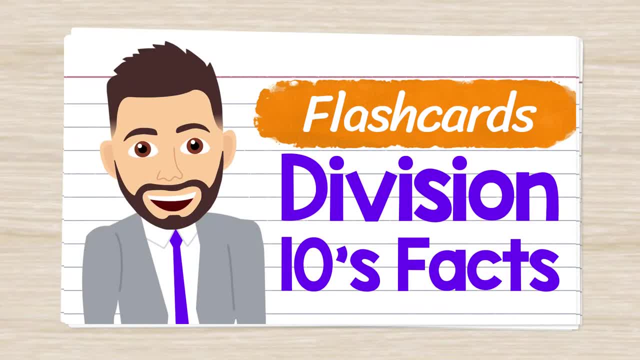 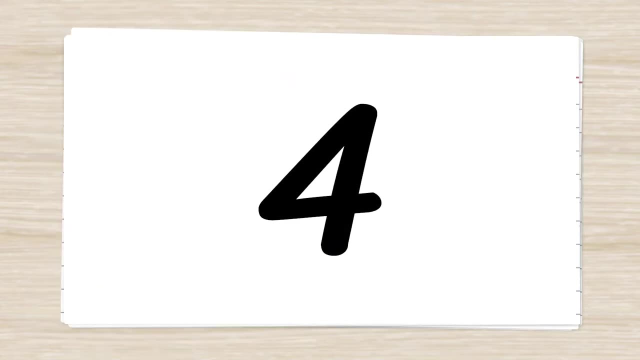 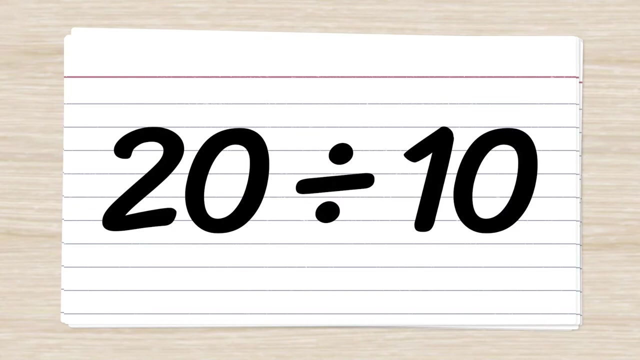 Welcome to Division Flashcards with Mr J And in this video we're going to go through the tens division facts. I hope you're ready. Let's get started. 40 divided by 10, 4,. 20 divided by 10, 2,. 70 divided by 10, 7,. 60 divided by 10, 6,. 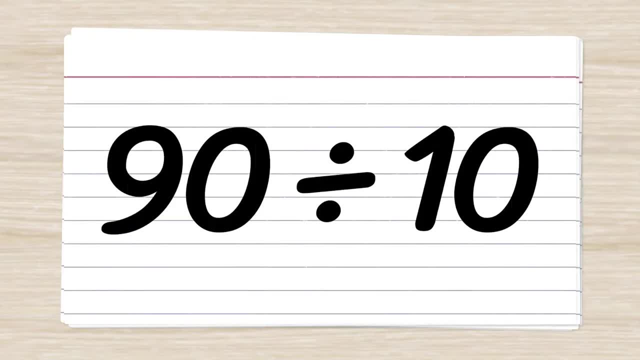 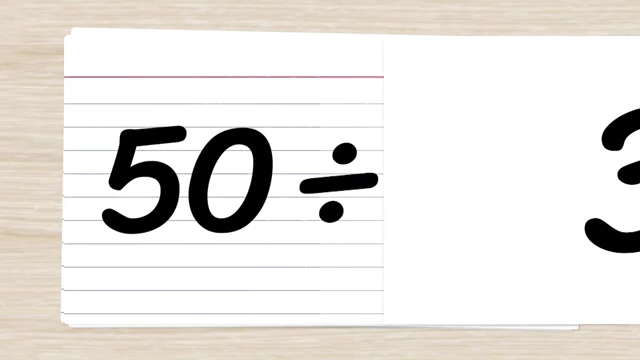 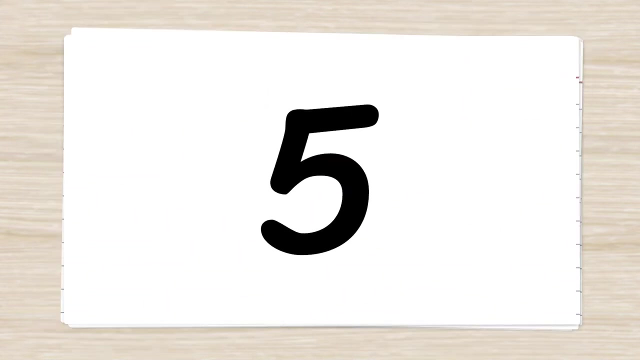 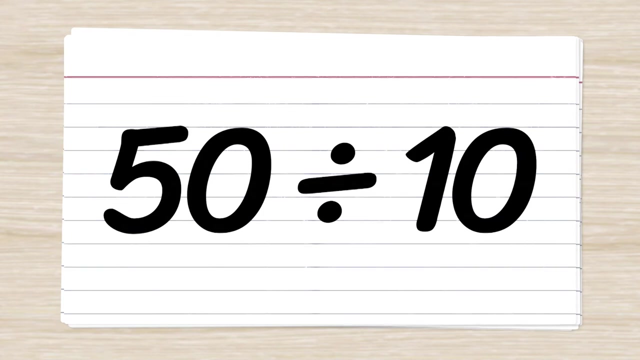 90 divided by 10,. 9, 30 divided by 10,. 3, 50 divided by 10, 5, 10 divided by 10,. 1, 50 divided by 10, 5, 80 divided by 10,. 8, 60 divided by 10, 6, 20 divided by 10,. 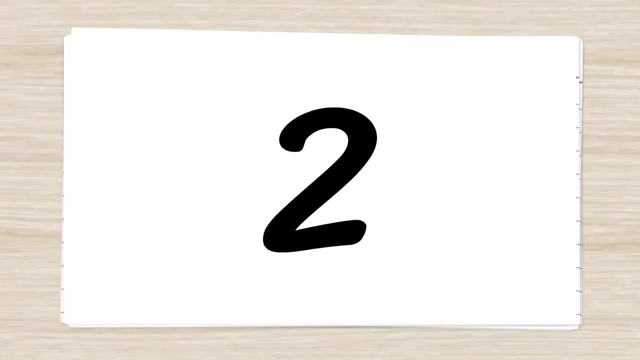 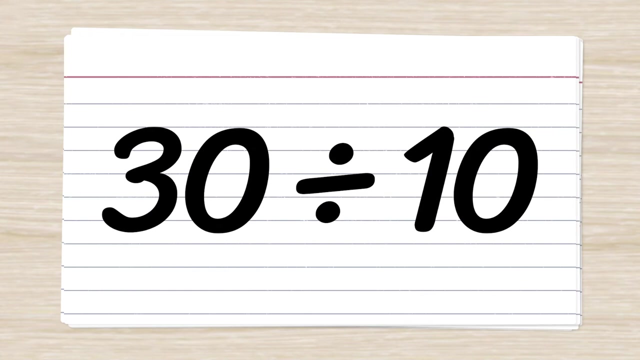 1,, 2, 80 divided by 10,, 8,, 30 divided by 10,, 3, 50 divided by 10, 5,, 7,, 7,, 8,, 9,, 10,.